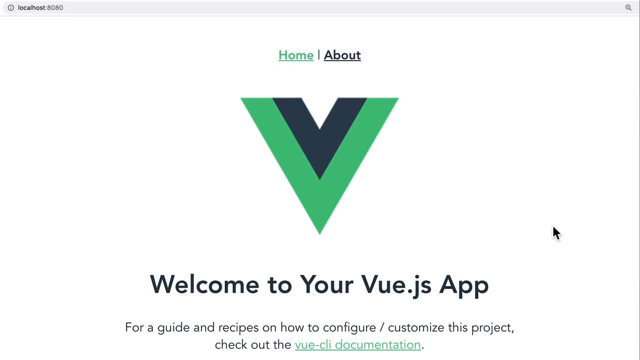 Notice there are two links up at the top. These links are used to navigate between the components in the source views directory called homevue and aboutvue. When I click the about link, Vue Router loads up my about component, and when I click home. 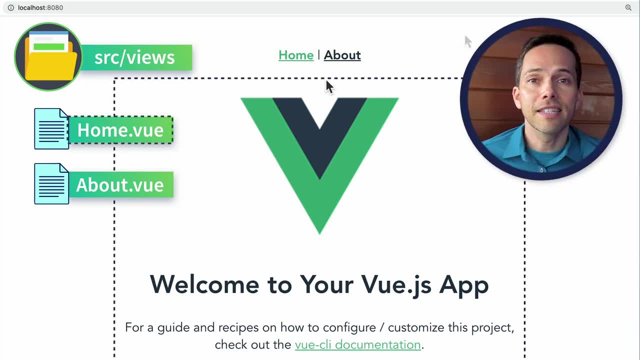 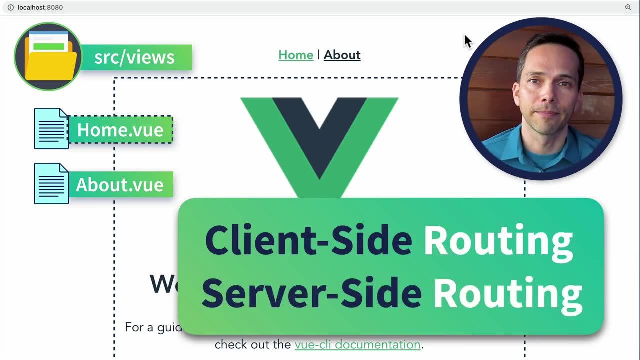 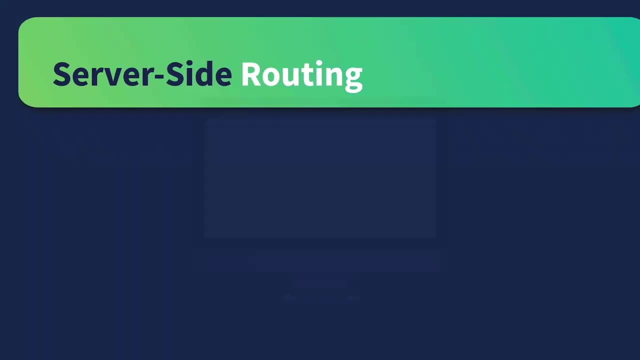 Vue Router loads up the home component. This kind of routing is called client-side routing and it's different than the older and more traditional kind of routing called server-side routing. By understanding the differences between the two, we can build highly dynamic user interfaces. 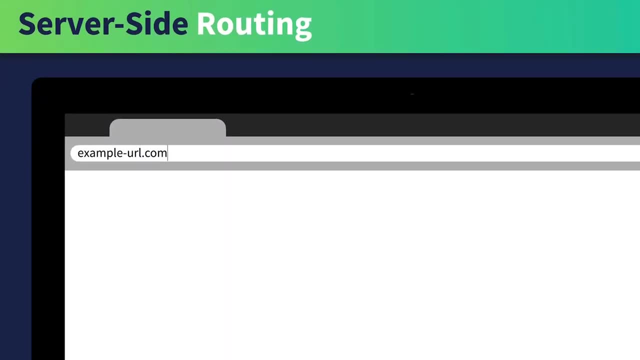 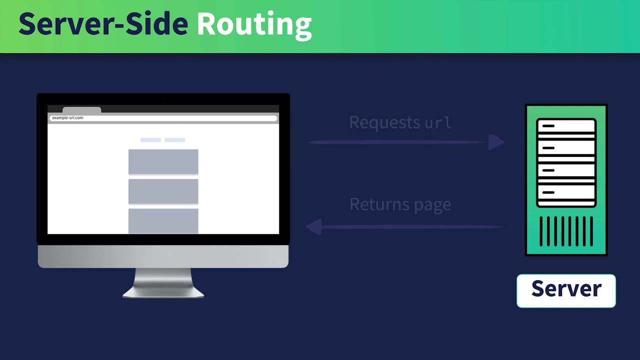 With a traditional server-side routed app. if a user types in a URL, the browser requests the URL from the server and the server returns the page. If the user were to click a link on that page, the browser would request that URL and return. 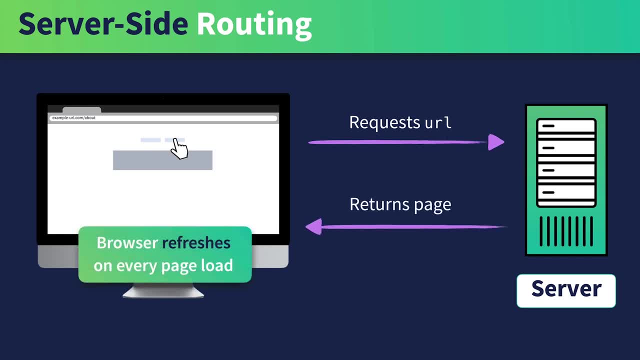 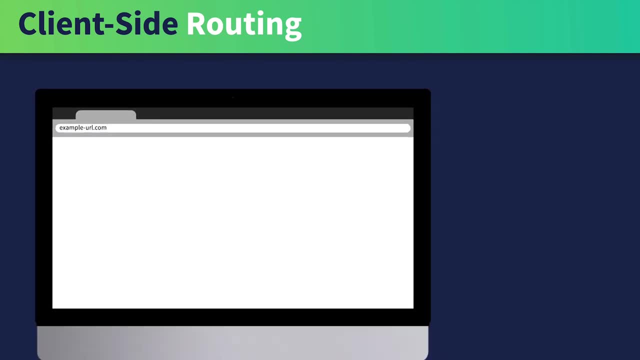 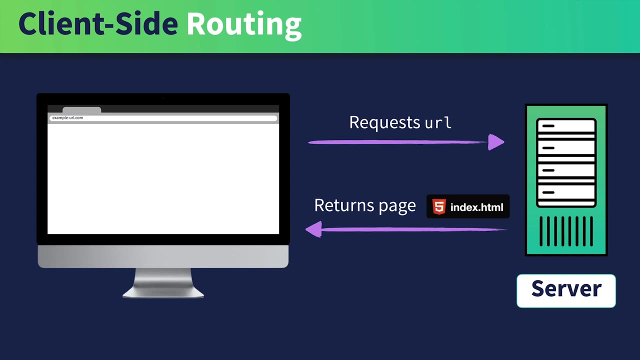 the new page refreshing on every page load. On the other hand, client-side routing looks a bit different. When the user types in the URL, the browser is going to request that URL and in this case the server returns that page, specifically indexhtml, which we'll touch on in just a. 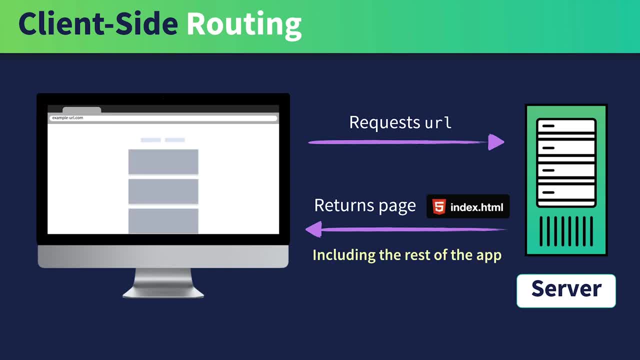 moment, and it sends along with it the rest of the app, Since the app already has all the code that it needs within the browser. when navigation happens, Vue, with the help of Vue Router, compares and renders the differences without ever having to reload the page. 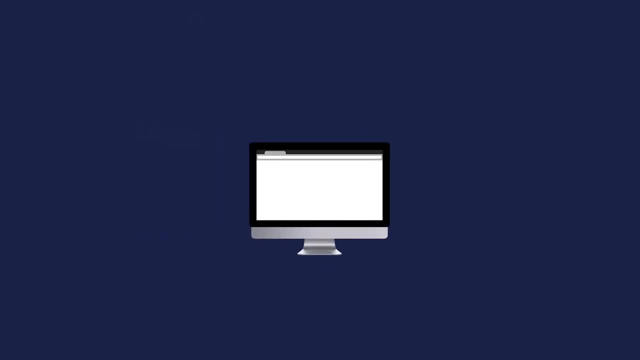 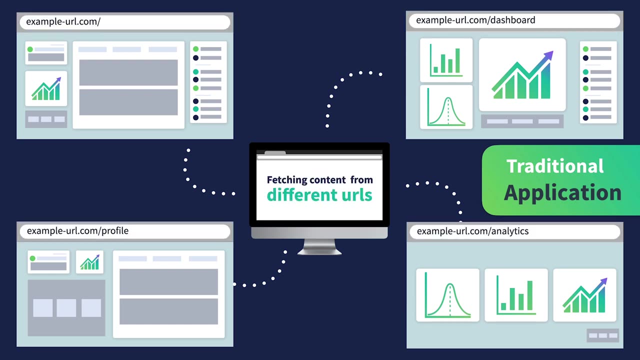 We can also visualize the differences between these two kinds of routing like so: In a traditional app that is not using client-side routing, the browser is essentially going out and fetching the different content that we need from those two types of routings. In a traditional app that is not using client-side routing, the browser is essentially going out and fetching the different content that we need from those two types of routings. In a traditional app that is not using client-side routing, the browser is essentially going out and fetching the different content that we need from those two types of routings. In a traditional app that is not using client-side routing, the browser is essentially going out and fetching the different content that we need from those two types of routings. 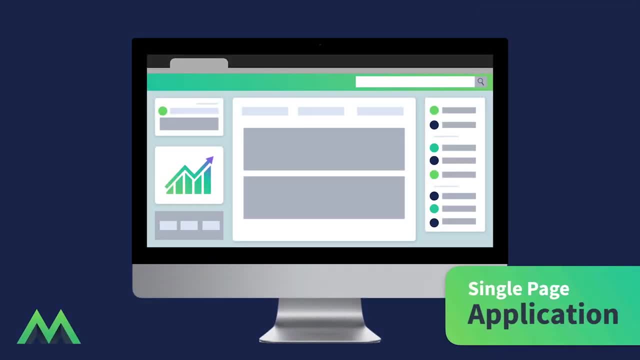 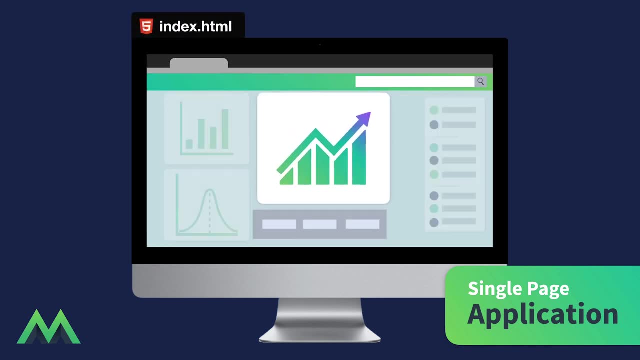 On the other hand, within a single-page application, we're really only looking at one page, the indexhtml, and as we click around in it we're adjusting which Vue we're seeing of that app. Hence we call it a single-page application, because all of these pages come from that. 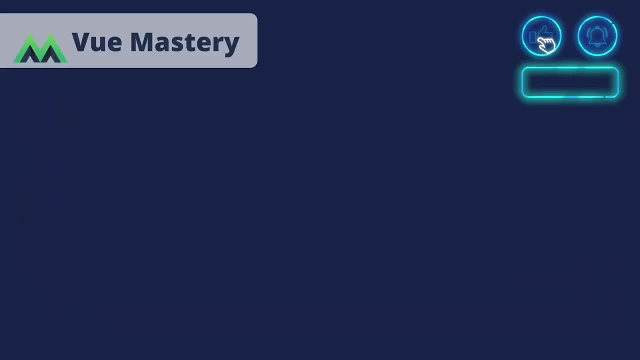 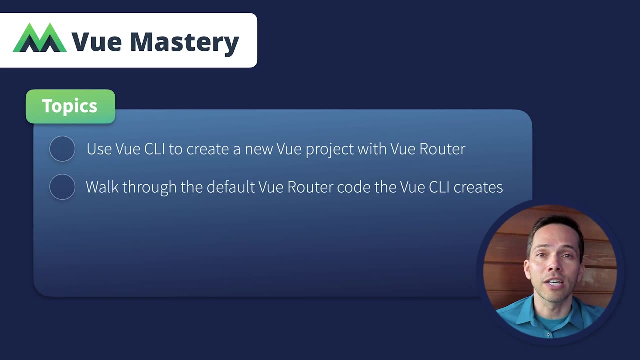 one indexhtml page. In the remainder of this video, we'll use Vue CLI to create a new project with Vue Router. We'll then walk through the code which is generated within Vue to gain a greater understanding. We'll take a glimpse at some of the most powerful features of Vue Router. 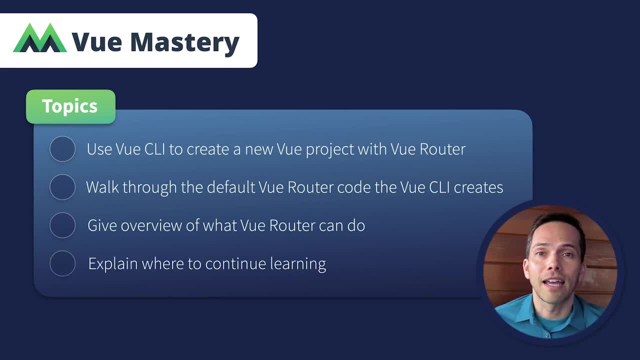 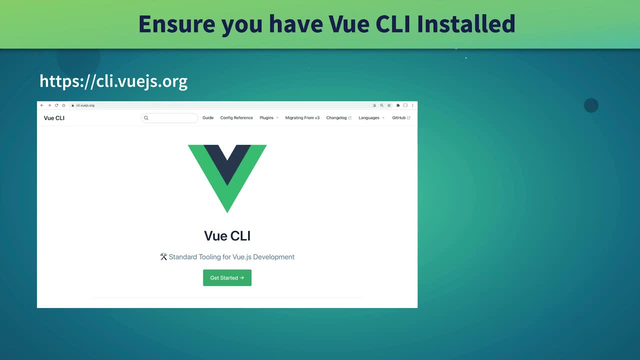 and I'll show you where to continue learning. There are a few ways to add Vue Router to a Vue project. We're going to start by using the Vue CLI, and I encourage you to follow along. First, I'll create a new Vue project by running Vue Create Demo. 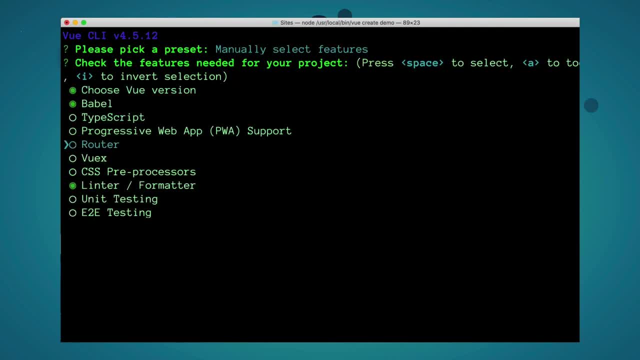 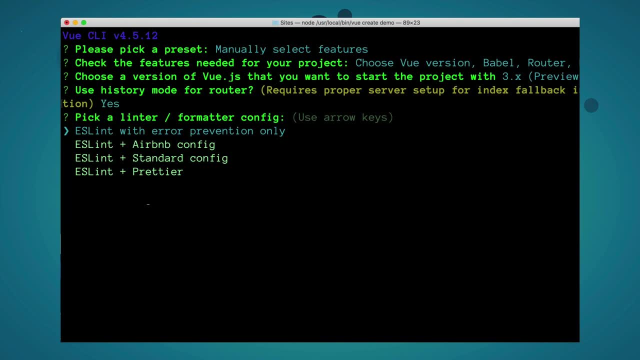 I'll select Manually. Select Features, Hit the spacebar to select the router and then hit Return. I'll choose Vue 3.. I do want to use History Mode, so I'll hit Enter. We'll use the default linter. We want lint onSave, so I'll hit Return. 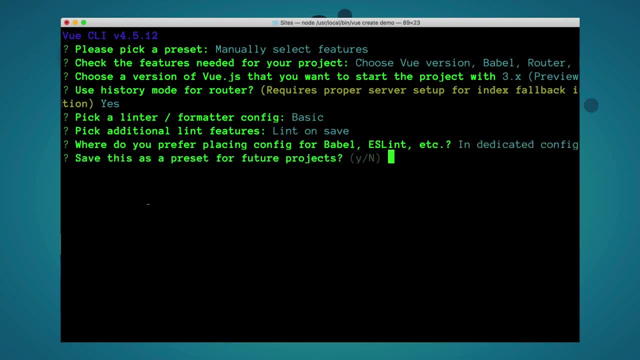 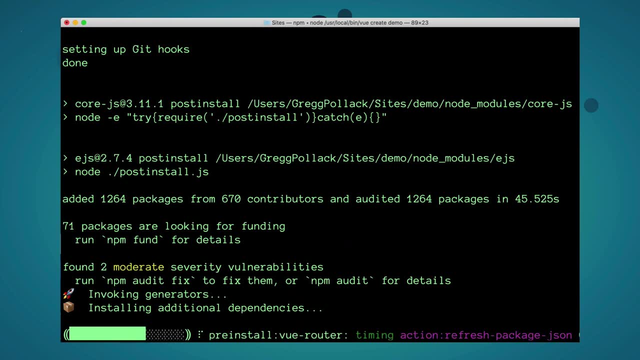 Dedicated config files are fine, so I'll hit Return And then I'll hit No for saving this as a preset. This is going to go create our project, run npm, install and now we can go into our demo directory and run our server. 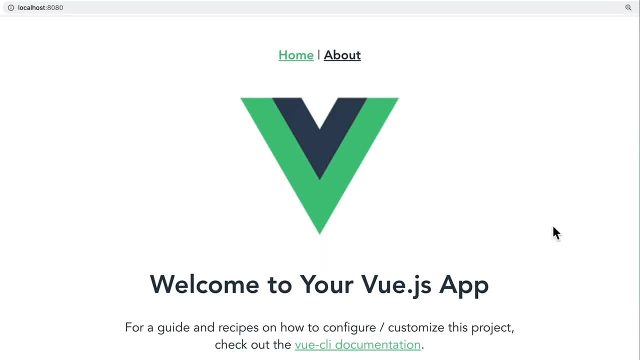 Great. This brings up the screen we've seen once before. Notice the two links on top. This is where we navigate between our Home and our About components. So when we click on the About link, Vue Router loads up the About component, And when I click Home, Vue Router loads up the Home component. 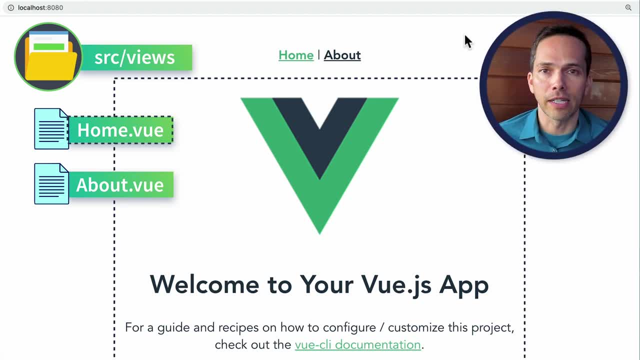 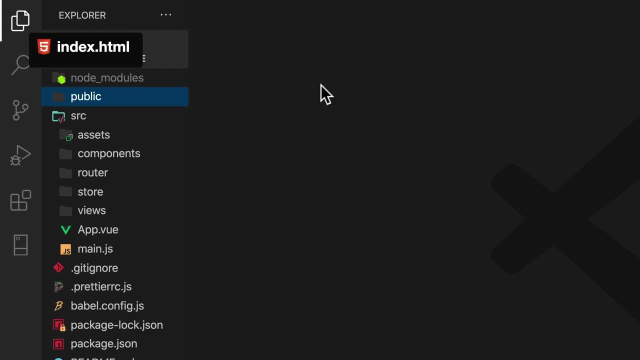 Now I'm going to hand you over to Adam Jarr, another instructor at Vue Mastery, to dive into the code. If we take a look at the project that was generated for us by the Vue CLI, we can examine the indexhtml file. 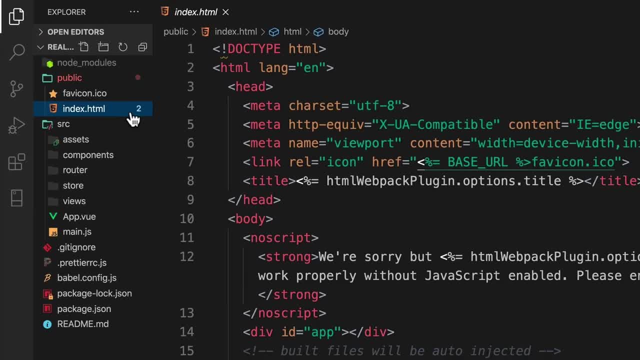 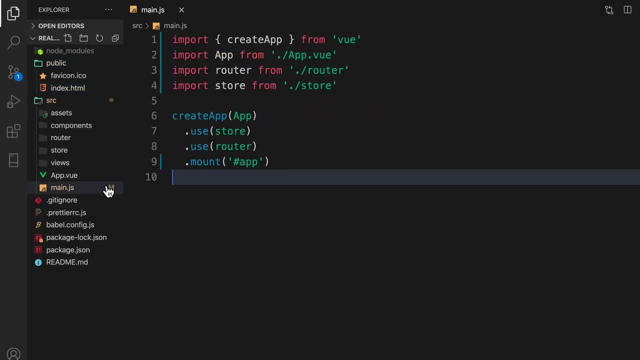 It's in the public directory and on line 14 is this div with the id of app. This will start to make more sense if we look inside the mainjs file, Inside of here, our app component, which is the root component of our entire application. 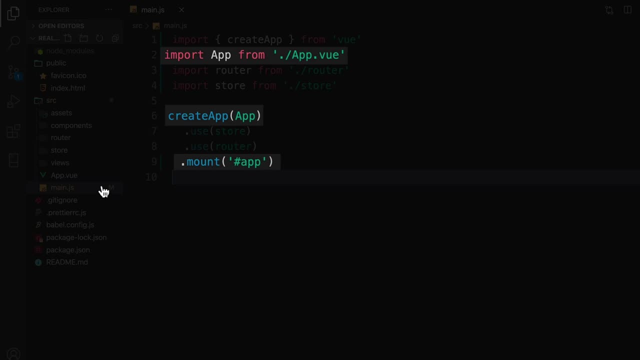 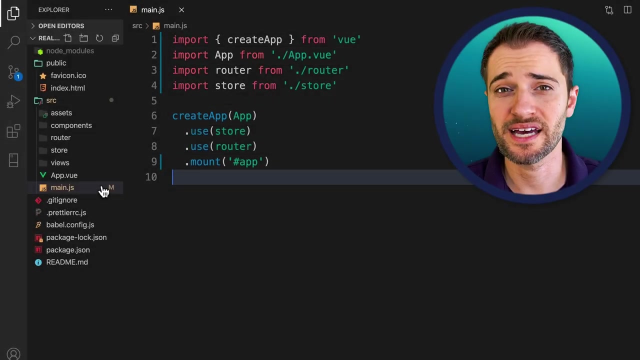 is being imported and used to create the app. It is then mounted to that div with the id of app inside the indexhtml file. So again, our entire application lives at that single page Indexhtml. Also in this file we're importing the router. 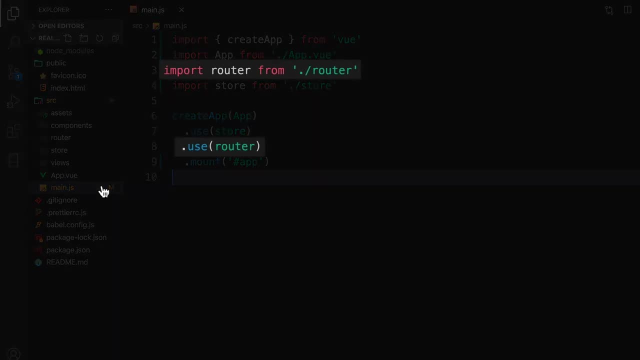 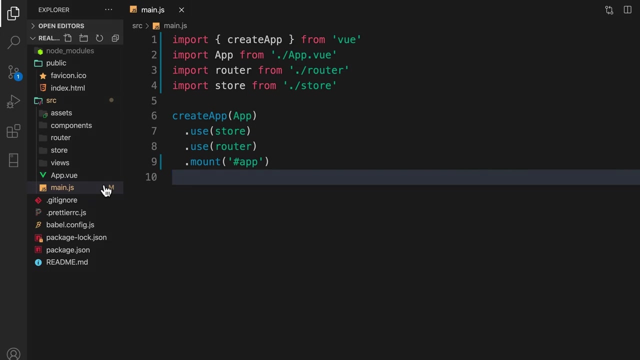 and when we create the app, we're telling our app to USE the router. So let's take a look at the router file to understand how it's all configured. Inside the router directory it has this indexjs file and you'll notice at the bottom we're exporting Router. 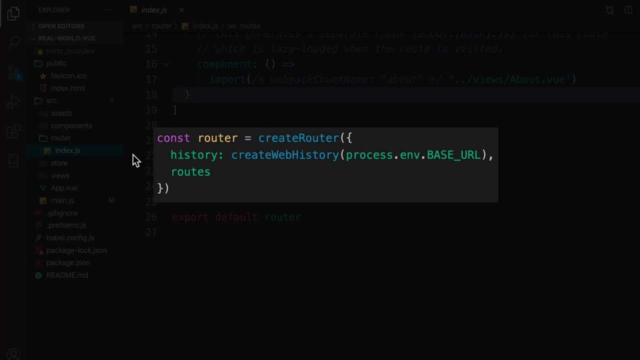 Just above. here we're creating the router and notice how we have this History property. When we created our plot, we were able to find the file. When we created our project with the Vue CLI, we selected to use history mode. That's why we're seeing this property here. 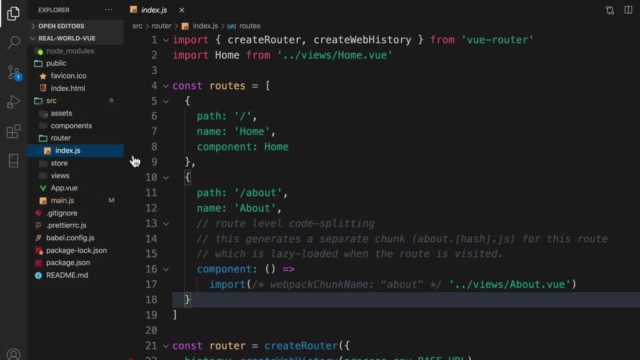 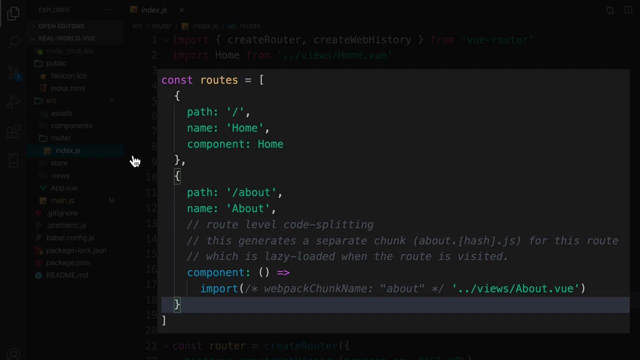 Also, here we're passing in the routes, so let's take a look at these. As you can see, we have a routes array with two route objects within it, Although they look a bit differently, which I'll touch on in just a second notice. how? 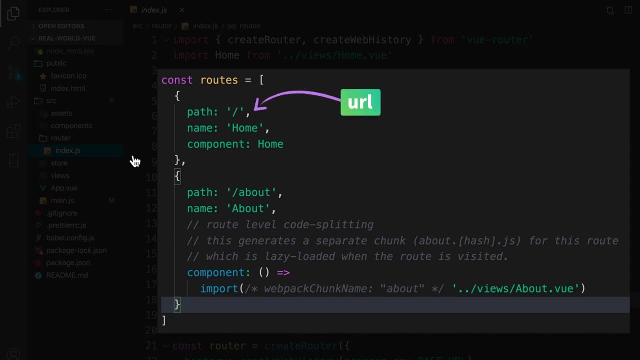 they each have a path, which is the URL for this route, along with a name and a property to specify the component to load when we reach this route. As you can see, we're importing the home component from our Vues directory. 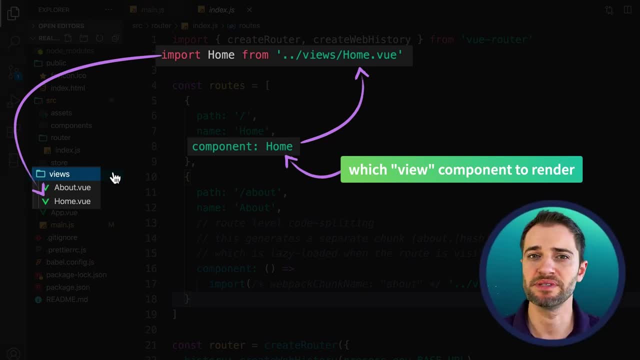 The Vues directory is where we put all those components that we want Vue Router to be able to load up as we navigate between the different pages. In this case, we have the home and about pages, each with their own route. Now that we have a basic understanding of how the router is configured, let's look 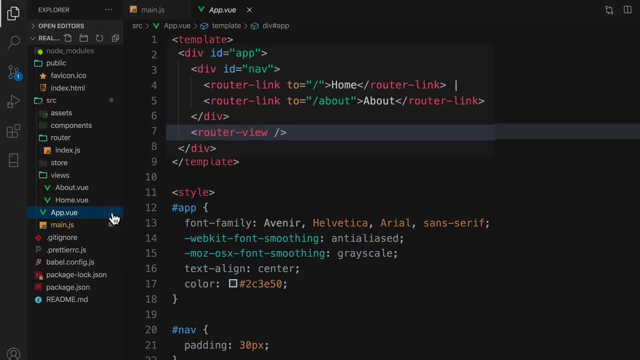 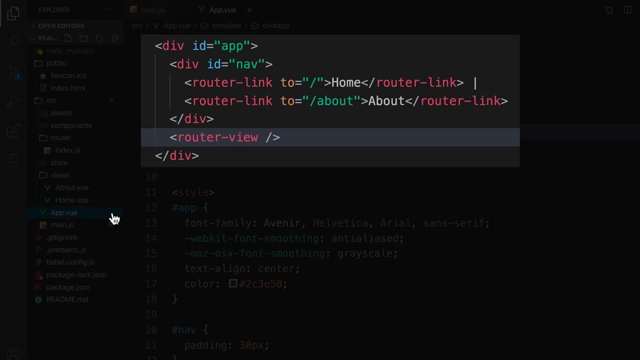 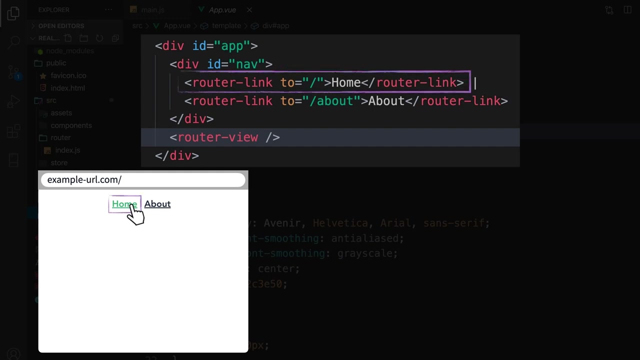 at how that site navigation is actually triggered. Notice here in the template there are these router links along with a router view component. These are built-in components. These are the components provided to us by Vue Router. When a user clicks on this home link, they're actually clicking on this router link here. 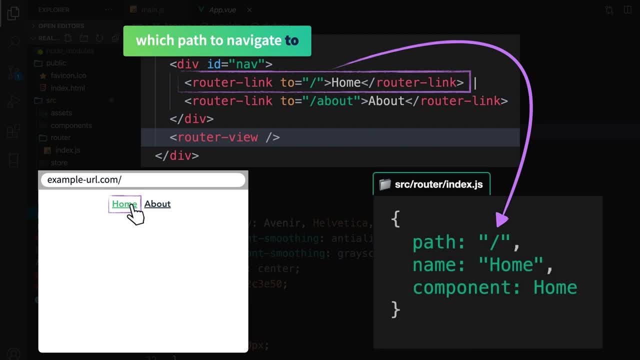 which has a to attribute specifying the path that we want to navigate to And when we navigate to that path because of this route object. here, Vue Router knows which component to load up. In this case, we're loading up the home component, but where do we put it? 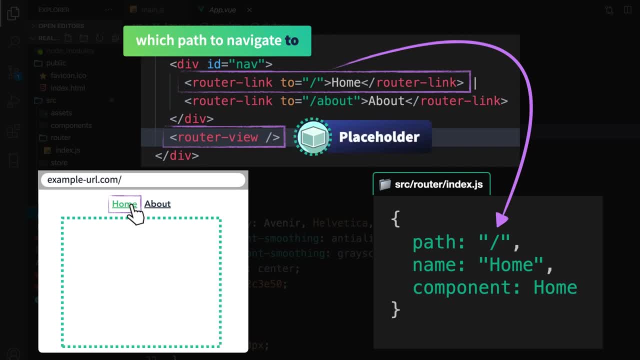 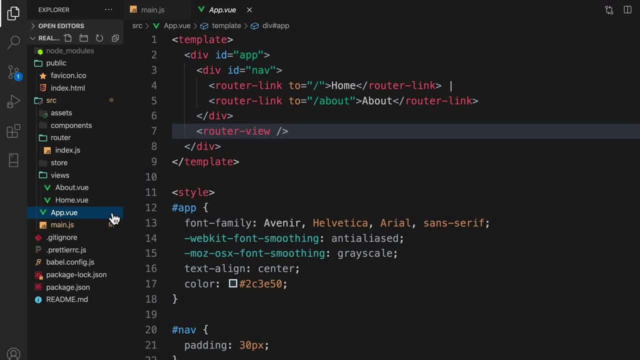 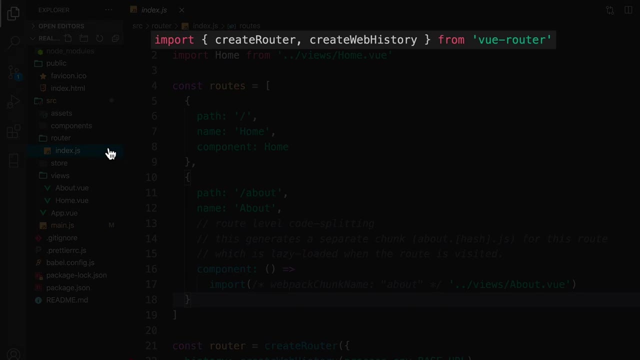 That's where the router view comes in. This functions as a placeholder that is replaced by the router view. We can also see the route's actual component. If we take another look at the router's index file, we'll notice that create router and create web history are being imported from Vue Router.